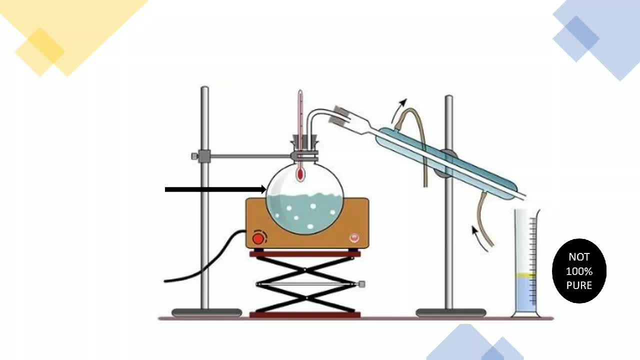 highly volatile and other is comparatively less volatile. what will happen when we heat the beaker or we heat the container? what will happen that the substance or the compound component which is which is highly volatile, which boils at low temperature, it will boil first and it will pass through the 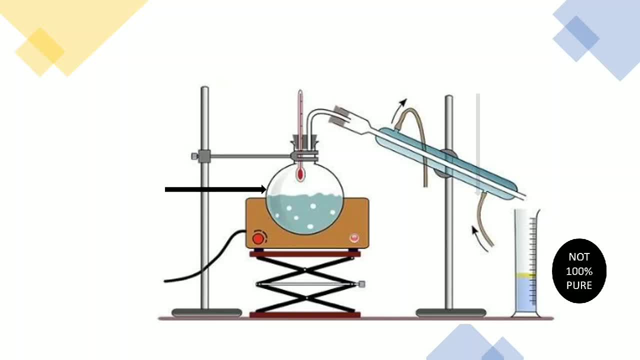 condenser. this tube with blue color around it is container, is condenser. all right, blue color shows the cooling water that is circulated around the condenser, So the vapors of the highly volatile component goes through the condenser. When it goes through the condenser it condenses alright and it changes its 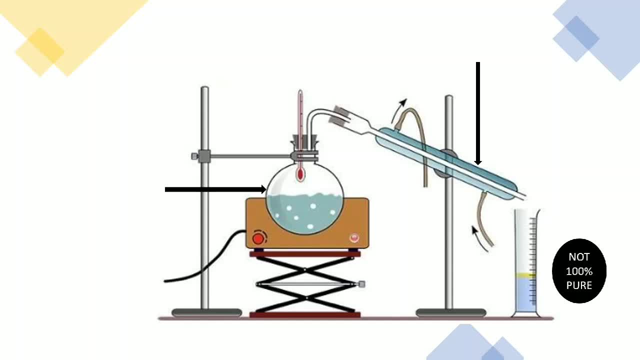 form, from vapor to liquid, and then we collect it into a separate container. But here we should note a thing: that the container, a separate container, does not include 100% pure component. When we heat the beaker or the container which contains a mixture of two. 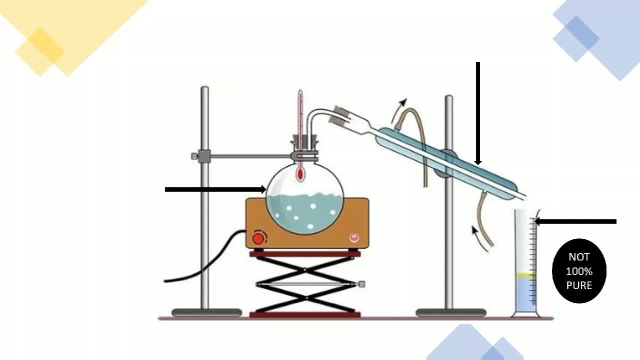 components- the highly volatile components- went through the condenser, but it takes some amount of less volatile component with it also. alright, But we get, we we will get- a larger fraction of highly volatile component. Now there are two laws on which 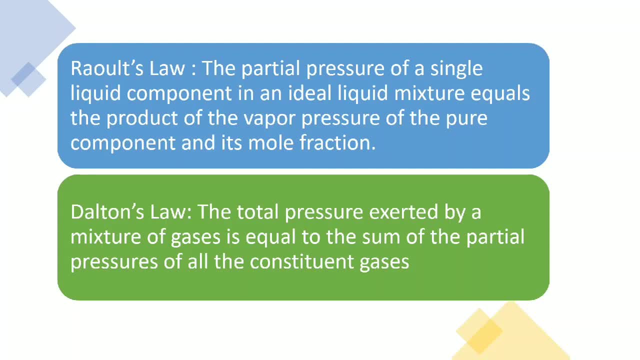 the distillation process is dependent on which are Raoult's and Dalton's law? You can read out the definitions here. When we heat the mixture of liquid, the vapor pressure of individual components increases, which in turns increases the total vapor pressure according to Dalton's. 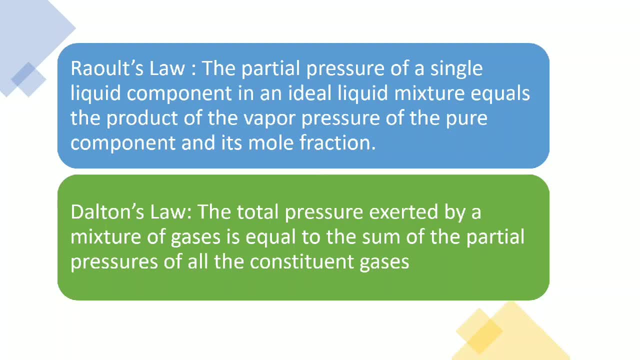 law. So so we can say that the mixture cannot have multiple boiling points unless the composition or the pressure changes During the process of distillation. the component with higher partial pressure is concentrated in the vapor and the component with lower partial pressure is concentrated in the liquid, But as we all know that in the mixture cannot the component. 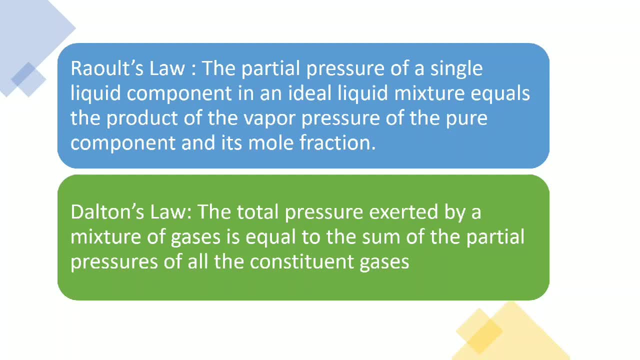 in the mixture cannot have zero partial pressure, So it is impossible to obtain a completely pure sample of a component from a mixture through distillation. However, a sample of high purity can be obtained when one of the component in the mixture has partial pressure which is close to zero. or we can say that 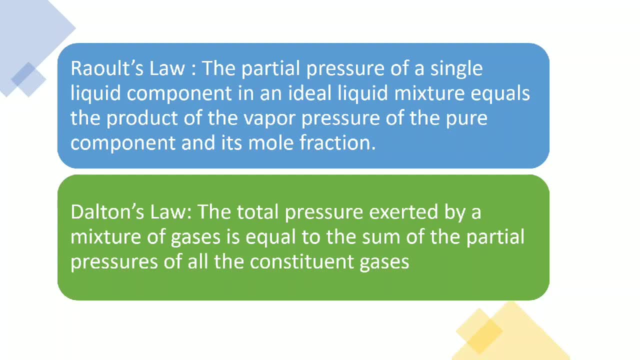 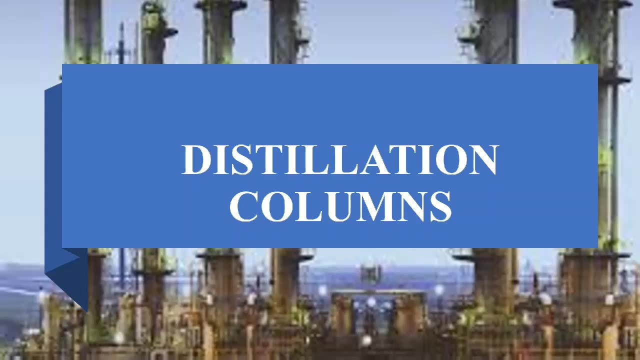 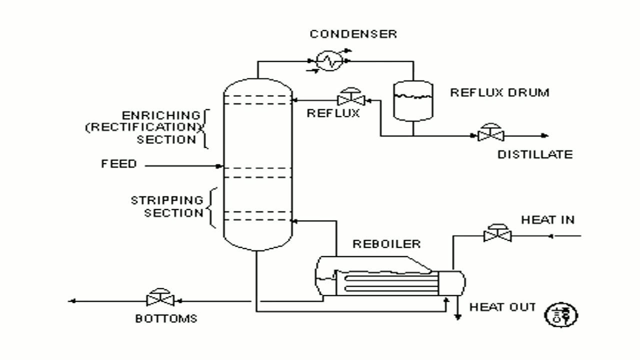 it is somewhat equal to zero. Now let's move towards the distillation column. It contains a vertical shell where separation is carried out and it is not totally disposed of. So we get all this vapor and its vapor is carried out. Then it contains the internals, such as trays, plates or packings, which is used. 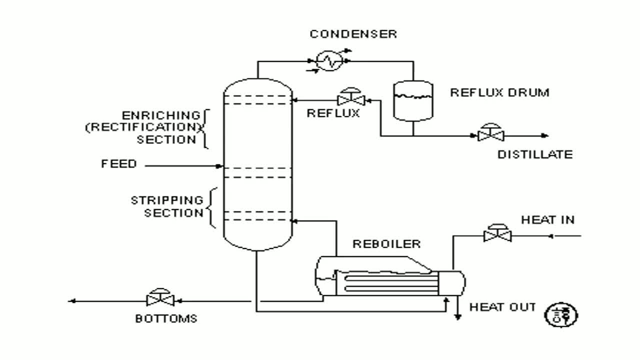 to increase the contact time between vapors and liquid. Then there is a stripping section, which is the lower section, which contains a reboiler to provide the necessary vaporization for the distillation process. Then it contains the enriches or rectification section, which has 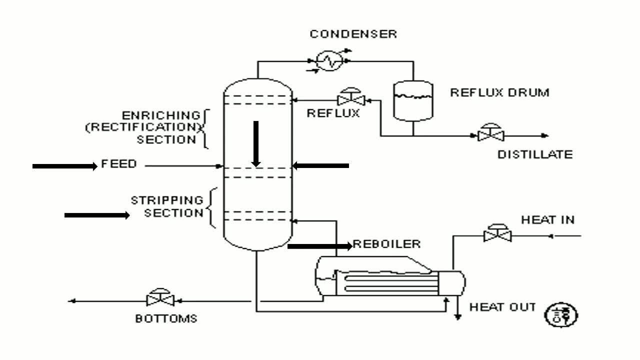 a condenser to cool and condense the vapor, leaving the top of the column, Then reflux drum to hold the condensed vapor from the top of the column so that the liquid can be recycled back to the column, and then the top and bottom products, which is known as distillate and bottoms. Now let's discuss. 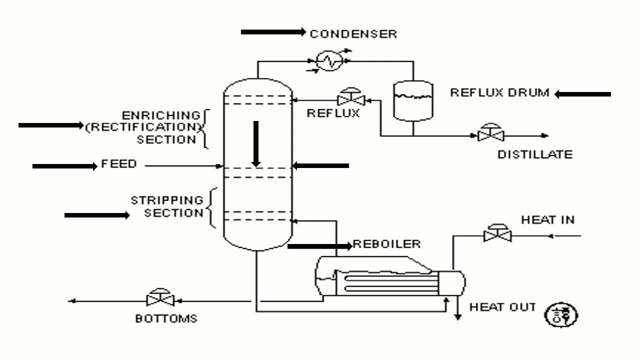 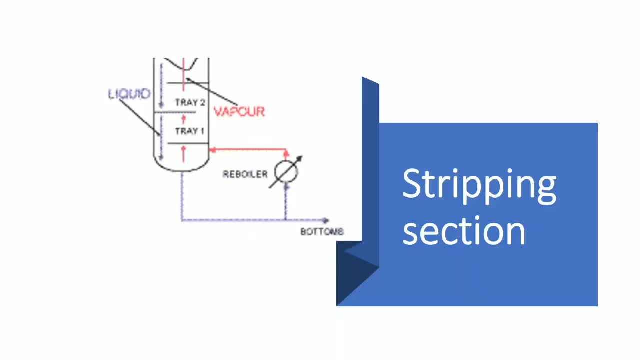 the basic operation or how separation takes place in our distillation column. So basically, feed enters somewhere in the middle- It is not necessarily the middle of the column, but it is introduced on a tray which is known as feed tray. Feed tray basically separates the two section of 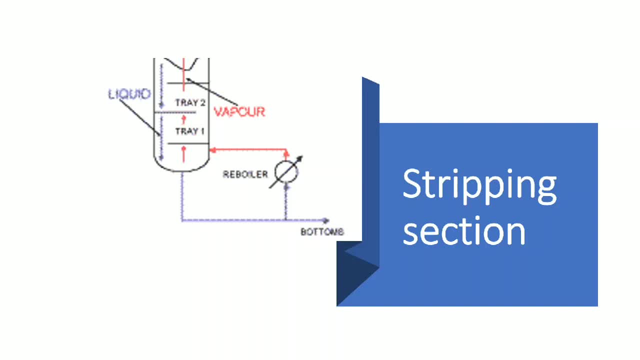 the column which we have discussed earlier, which is enriching or rectification section, the top distillation column. So basically, feed flows down the column where it is collected at the bottom in the reboiler and heat is supplied to the reboiler to generate vapors, The heat source. 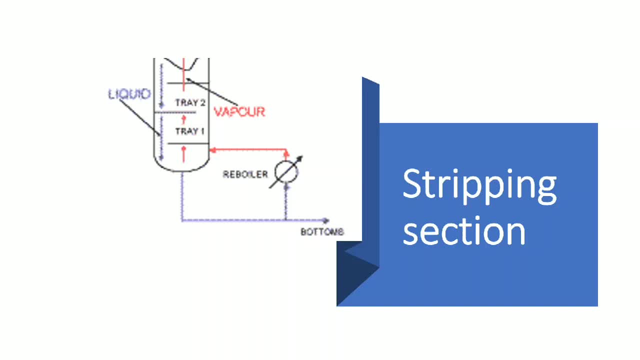 may be, anything can be. we can use anything to supply heat to the reboiler. but in most of the industries steam is used. All right, the vapor raised in the reboiler is used to generate vapor. The vapor in the reboiler is reintroduced to the unit at the bottom of the column, The liquid.